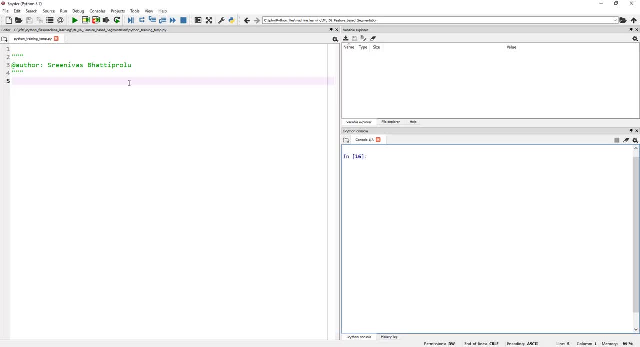 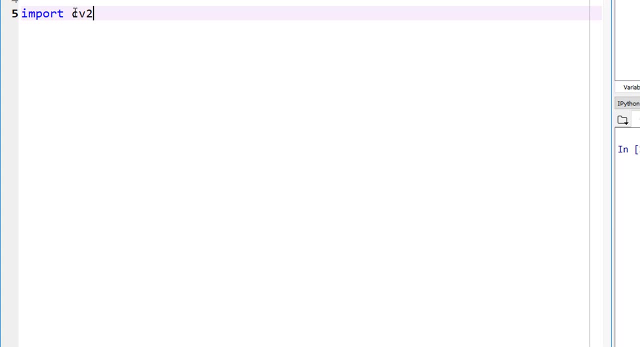 our code. So here is the spider interface And let's start, as usual, by importing our image. So I'm going to do import, I mean import the libraries to open the image. So import cv2, which is open cv, And let's assign our variable image as cv2.img. 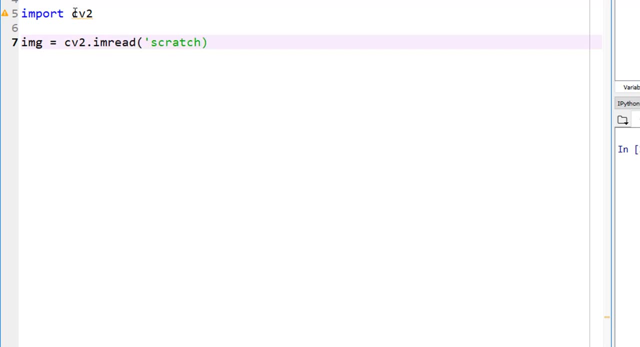 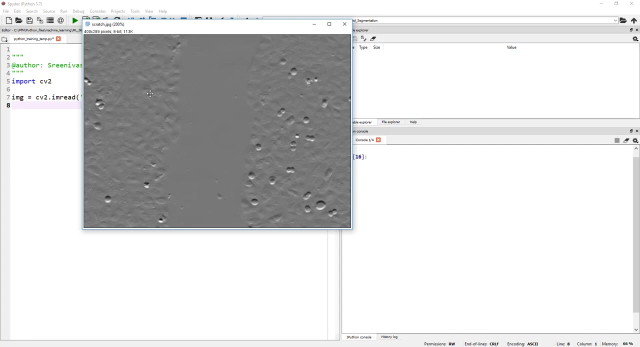 and I'm gonna import a file called scratchjpg. this helps me demonstrate one filter, for example. let me open the image right here so you can see. this is the image I'm trying to open and, as you can see, this is a tough image to segment using traditional histogram segmentation. obviously, as 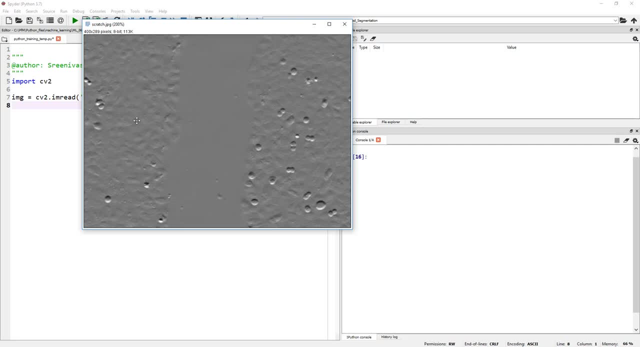 humans, we can see that this area has a lot of texture compared to this region, which is very flat. but how do we segment these regions? well, for that, a good filter- I mean you can use variance filter that can actually describe this region, but a good one that can really help- is called entropy. 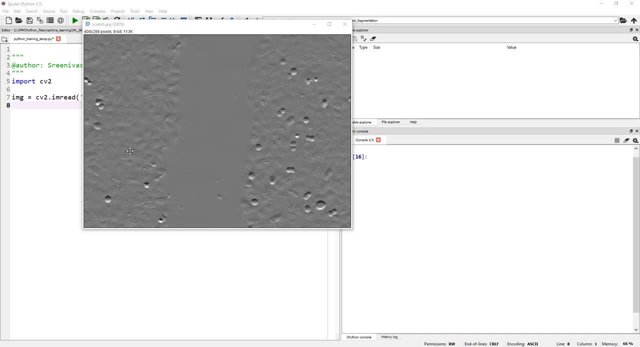 filter. yeah, if you have taken thermodynamics class in the past or any statistics class, you probably- or even just plain English definition, you probably know entropy as lack of disorder, or entropy is a not lack of disorder, lack of order, sorry, And entropy basically is a measure of. 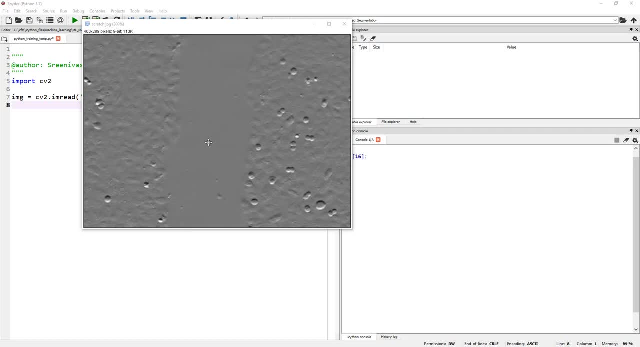 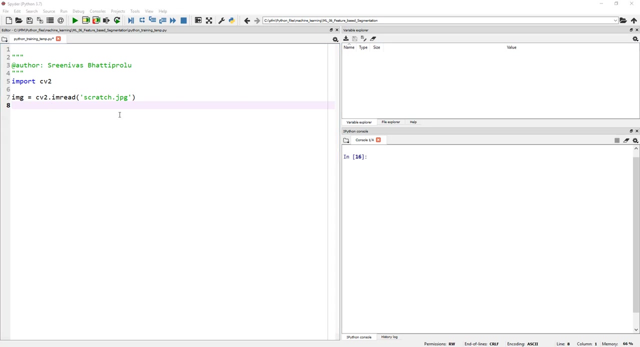 disorder And in this case, if you look at an individual pixel level, I see more disorder in this region than the flat region right here. So hopefully entropy filter is going to help us and the way we actually look at this. load this entropy filter. let's go ahead and import the right library. It is in SK image. 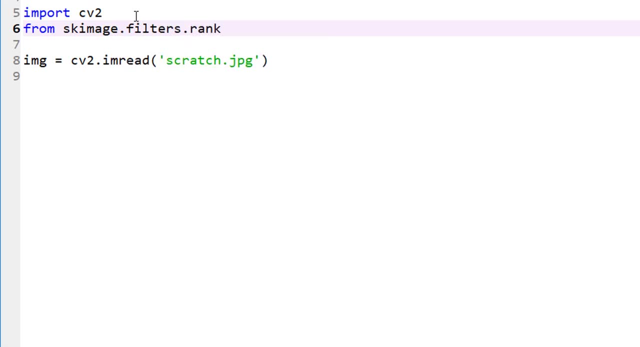 dot filters, dot rank and again. you can look at the documentation if you want. but entropy filter requires us to define a disk size because that's like the kernel size that we define. So that's also present in SK. image dot morphology. Okay, morphology. 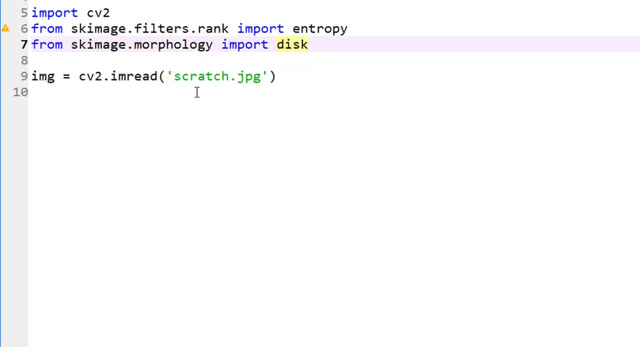 Import disk. Okay, and again, this is just one example. You don't have to use this one. This is just one example. There's so many filters out there. Go ahead and do some research As the subject matter expert. you need to understand. okay, what filter is the right one to describe the features in your image? 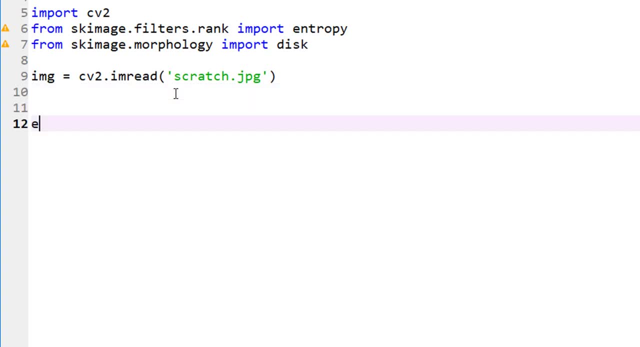 Okay, so that's pretty much it. Once I import that, I'm just going to say entropy, image equals. we imported entropy, right, So? and then the inputs are our image, okay, and disk size. And let's say disk size is one for now. Okay, and by the way, 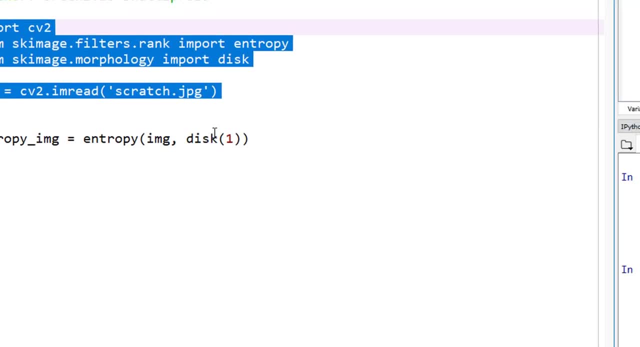 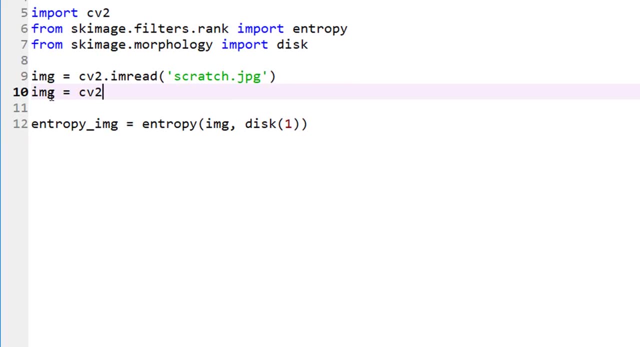 if I run up to here, I should see what my image is. It's a RGB image We can choose to. actually. let's actually convert this to single color. I mean gray level, CVT. Did I make a mistake Color? I think CVT color. Okay, so our input is our image and let's convert this to. 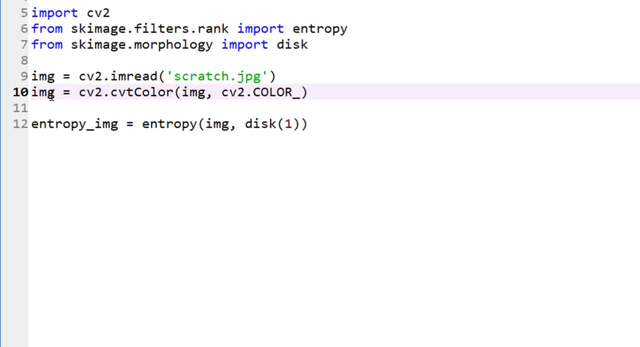 gray. I think it's underscore BGR. Again, remember, this is OpenCV, so it's not RGB, It's BGR2 gray. Okay, so just for the fun of it, let's run these lines to make sure we haven't made any mistake. 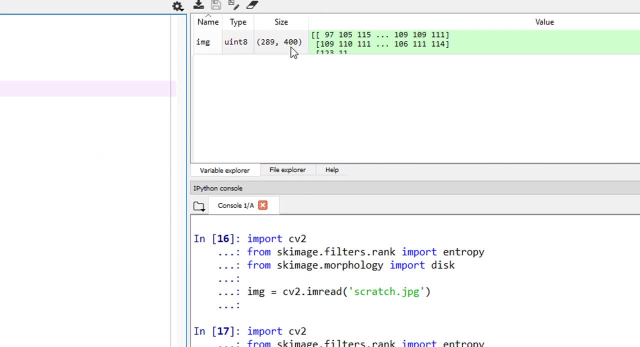 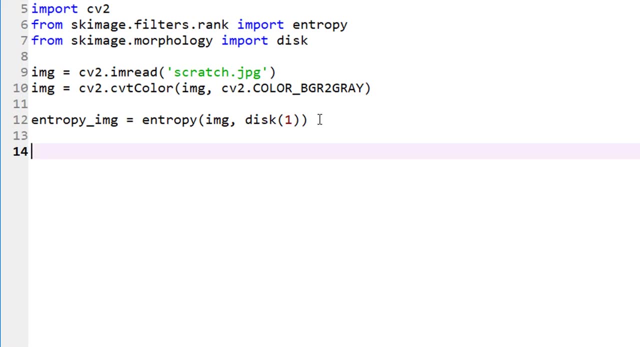 Everything works fine. My image is now only a grayscale. You can see the dimensions up here. So now I'm ready to come down and then visualize my entropy image. And how do we visualize this? CV2.imshow And my title is going to be entropy and the image name: 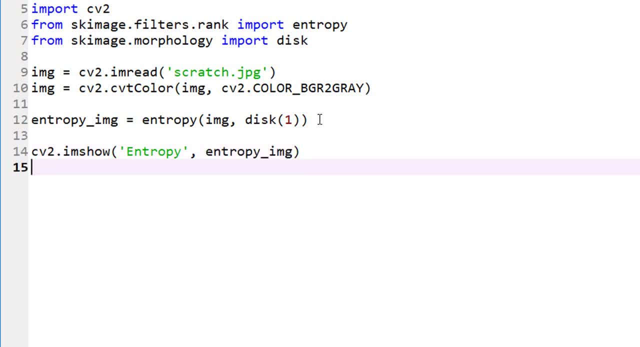 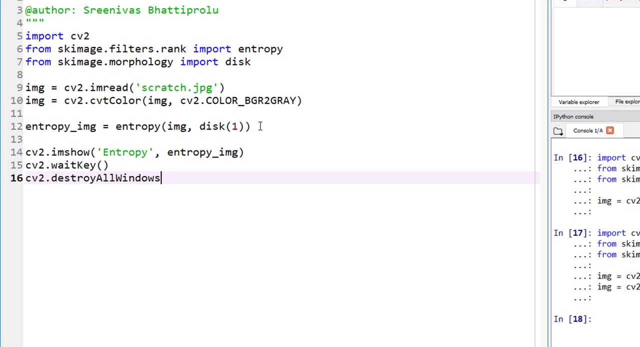 entropy: underscore image. Now do not forget to type this: CV2.waitkey- I-T-K-E-Y. You can provide how many milliseconds you want the image to be open right there, but after displaying the image, destroy all windows. Okay, so now let's go ahead and run this so we can see. this is how the output in fact. 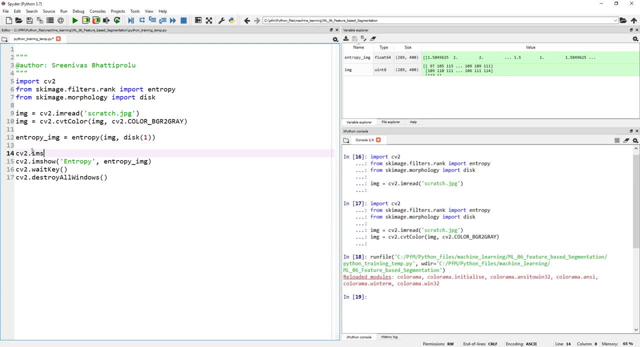 Let's go ahead and CV2.imshow original image. okay, So it's easy for us to compare and our original image is just IMG, right? Okay? so let's run this one more time. and here is the original image and here is the entropy image. 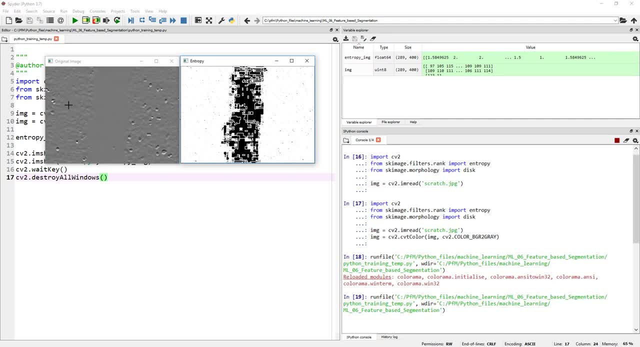 You see how we can use entropy values, Because here the value is very high. wherever we have disorder, wherever we have some sort of an order, you know the value is low. So entropy can define. entropy is one of the good features that I can pick to describe this specific image. 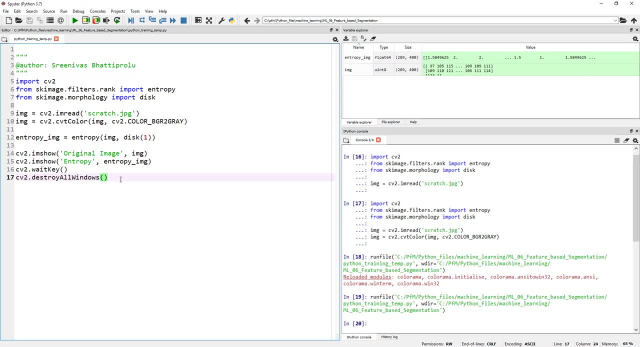 Okay, now what if I have a different image? and let's actually let me import. what other images do I have? I think I have an image called yeast cells. Again, these are the ones I just downloaded from the internet, png, and let's, let's go ahead and do this. 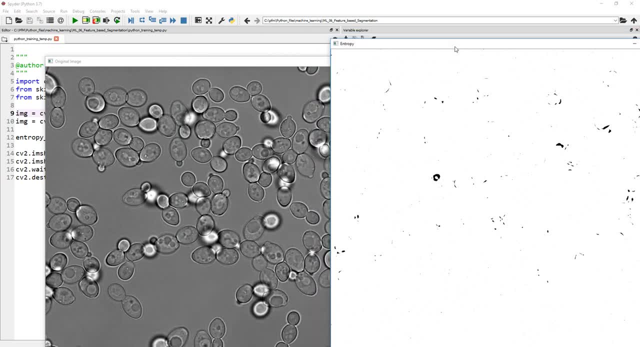 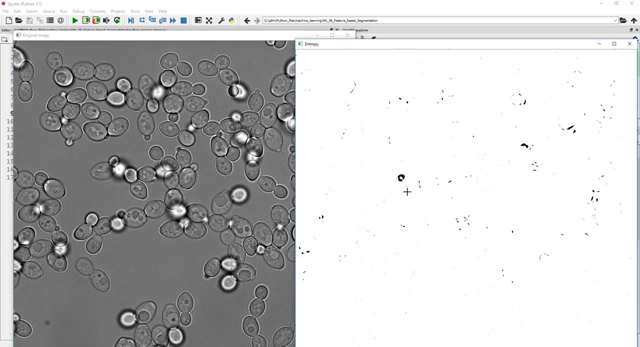 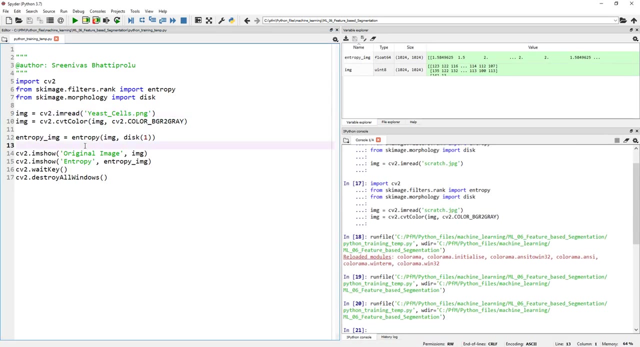 yeast cellspng. and here it is. So entropy is not a good filter to describe this, as you can see. So this is the original image and this is the entropy filter, and I see a bunch of nothing. So it tells you the importance of picking the right type of filters. So, in addition to entropy, what else should we select? 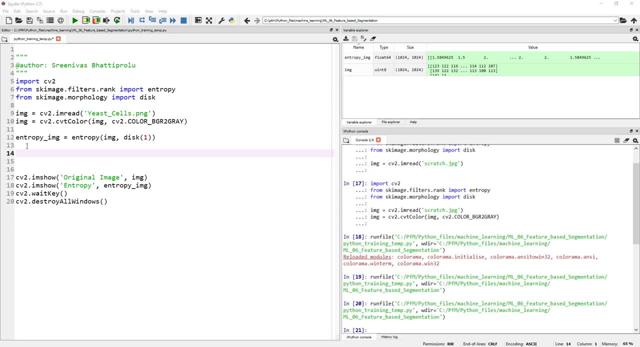 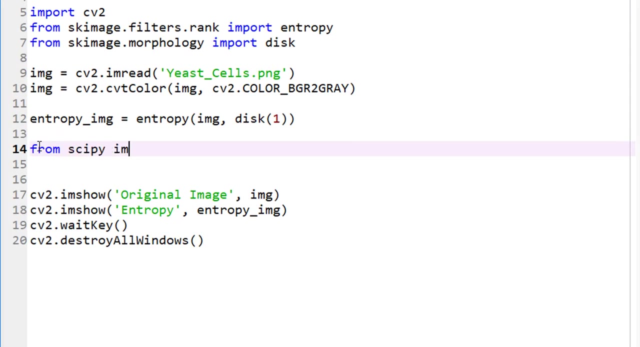 Let's do Gaussian blur. I mean just to show you. and Gaussian is, Where is the Gaussian filter I think it's part of? again, let me go ahead and import it right here from scipy: import nd image as nd. Okay, by the way, some of these filters are available in multiple libraries. 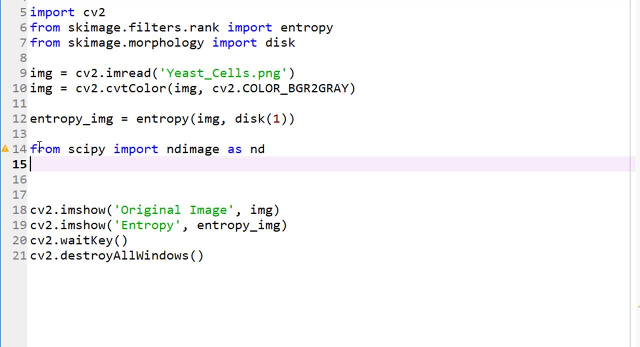 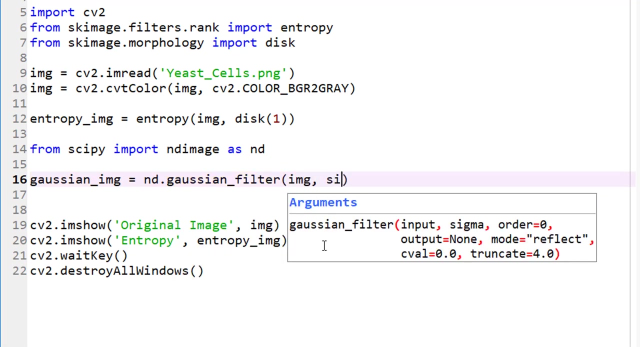 So use which one you think you know most of them should do a similar job. So go ahead and use whatever you think will do a good job or faster job. I should say sometimes Gaussian. my Gaussian image is nd dot. Does it show Gaussian filter? Yeah, right there, Gaussian filter and the arguments it takes is input, is image, and 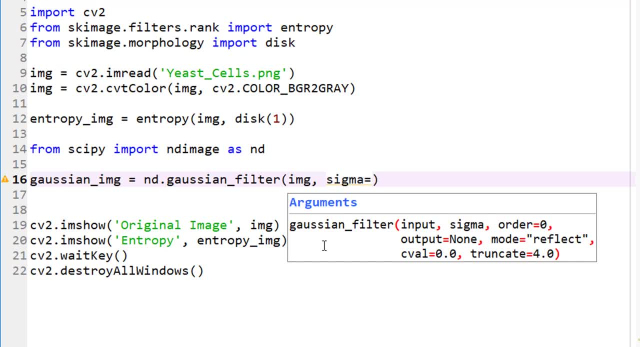 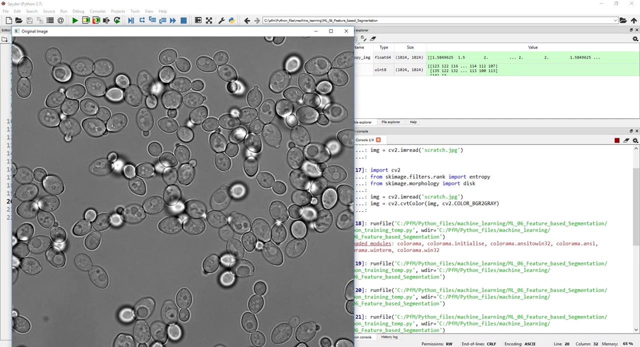 Let's put Sigma Equal to 3 for now. Okay, again, this is: the larger the value, the more blurry the image gets. Okay, so our Gaussian Right now is Gaussian underscore image. Okay, so let's go ahead and run this, and Here is my original image and here is my Gaussian image. and again, what is it describing? Well, we don't know. 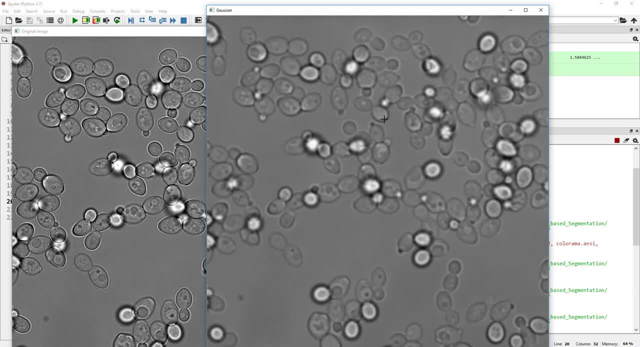 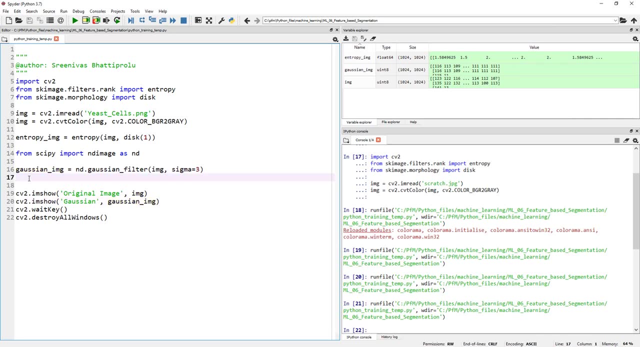 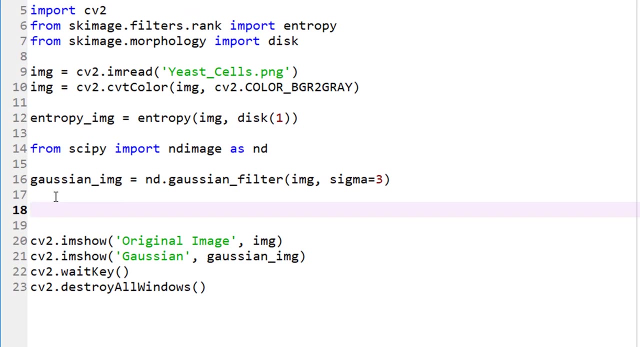 I mean, maybe this is useful, Maybe this is not useful for our machine learning, but this is another filter that we can definitely consider. and Let me just do one more before jumping on to, You know, creating a feature vector. so one more. so, Bell, I like this because it's a very good on edges. So, from 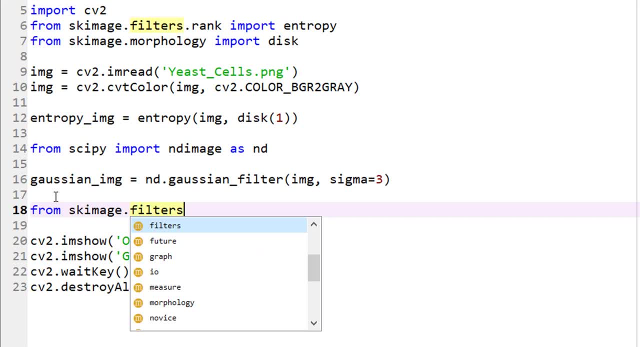 Escape image filters. There are a bunch of these. Go ahead and look at some of these filters. So, Bell? Okay, Now I'm gonna do my. so, Bell. underscore: image equals. That's it, Okay. so let's not use any math. So, Bell, and let's see how that looks like. 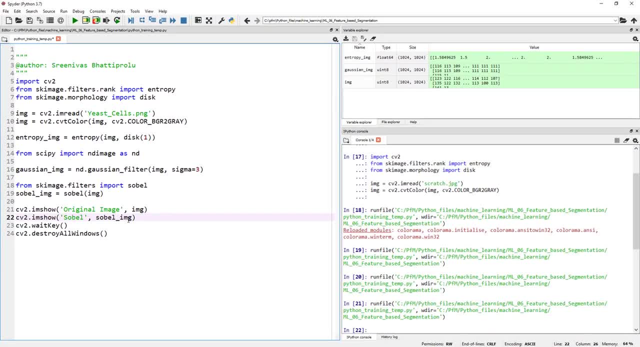 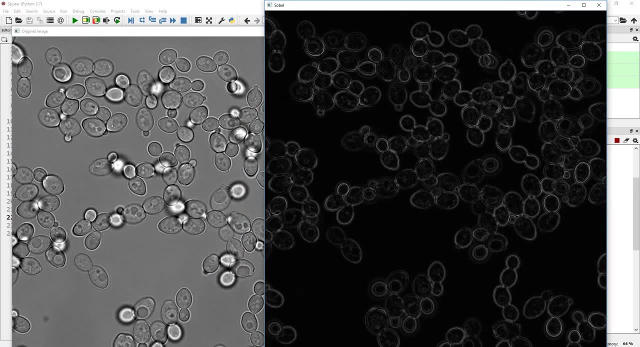 So Okay, so let me go ahead and run this and We should see there you go. So this is the original image and this is the edge. Well, are so Bell filtered image, which definitely shows us like all these regions with hard edges. So this can be a very good filter to separate the cells in this image. 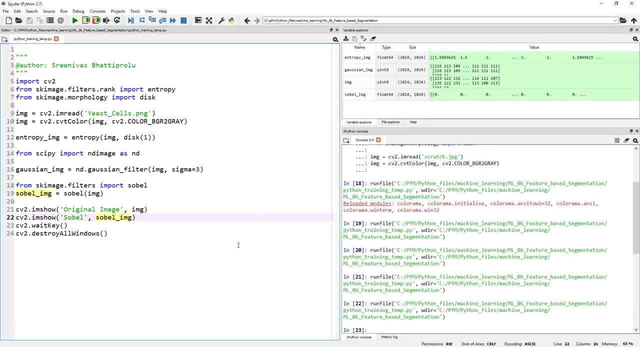 okay, so now I hope that you understand how to extract various filters. I can literally do this lecture for another hour to show every little filter that there's out there, but then look at documentation under SK image filters and also other documentation. you know for image filters, but this is how you can. 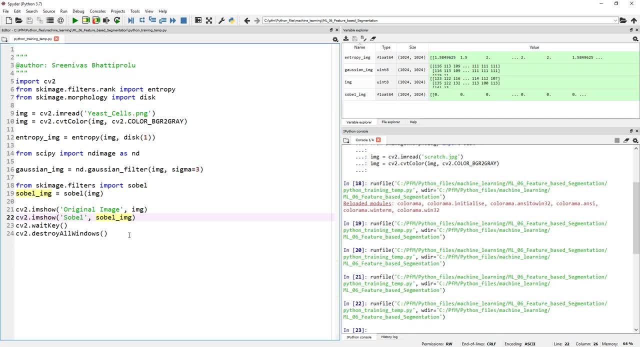 actually generate these filters, but how do you put all of this information together to create, like a pandas data frame that we can use as input into our machine learning algorithm? yeah, so for that. let's again, let's do this in a methodical way. okay, so let's start in the 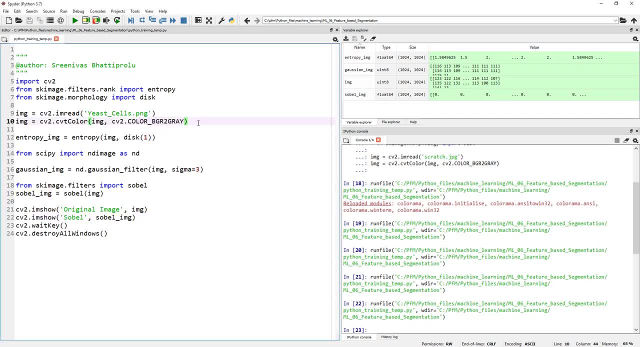 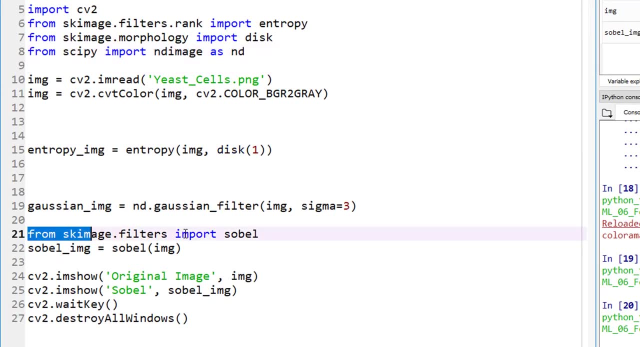 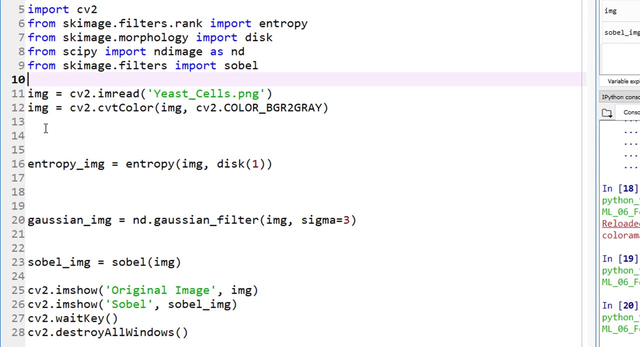 beginning right there. okay it. things can get confusing if we are not careful. let me move these libraries up here. okay, there you go. let me move the libraries up here, and the first thing we do is, of course, read our images. and now for pandas data frame, where we can. 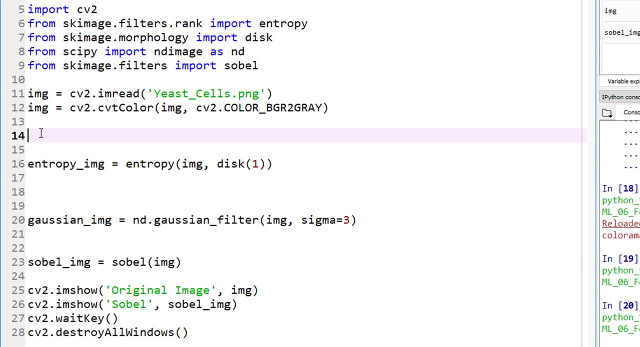 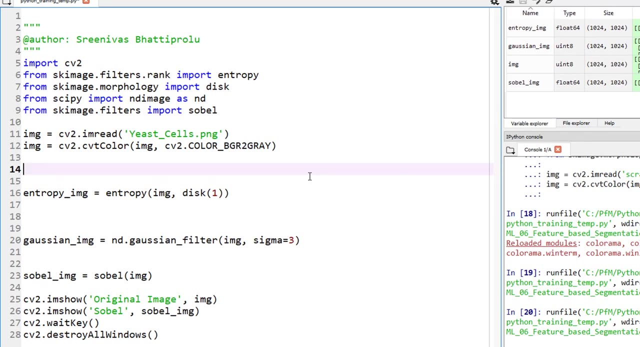 actually create these feature vectors. it helps well. in fact, it's almost required for us to convert our 2d image. you see, our image here is 1024 by 1024, right? I want to convert that into one single list, you know where, or one single array, if you want to call that so, which means: 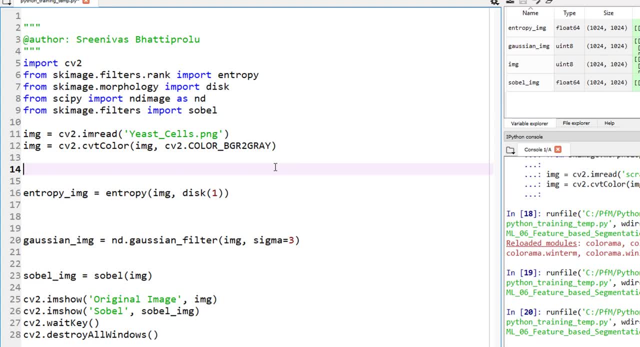 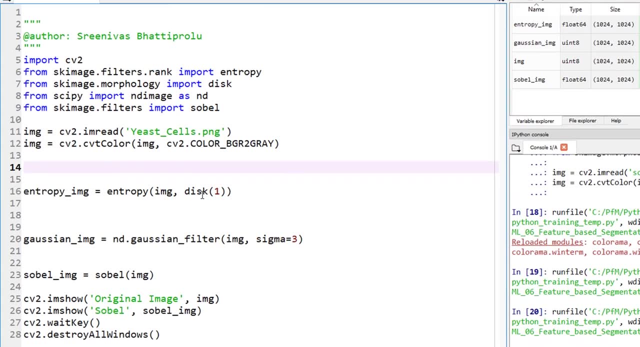 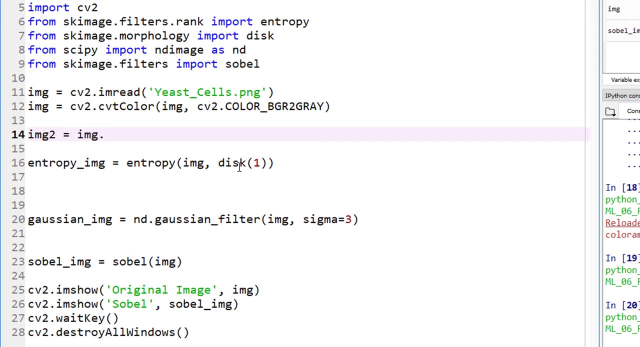 I'm going to unwrap my 2d image into one dimensional array. okay, and we all know again, hopefully, if you watch my previous video- how to do that. so it's nothing. but image 2, okay, equals image dot. I mean, image 2 is just a name I gave like image dot, reshape. okay, minus 1, so that's just a shortcut. 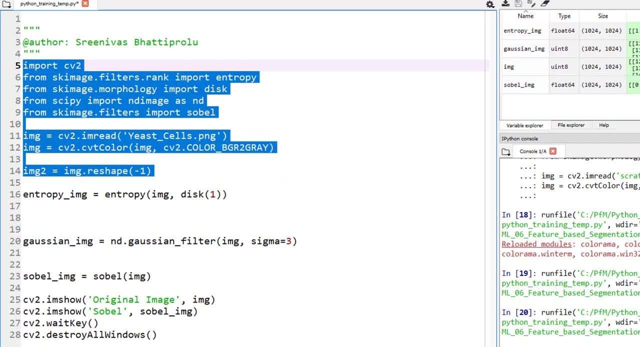 to say: okay, convert that into single. so let me go ahead and run this so you can see how my image 2 is nothing but 1, 0, 4, 8, 5, 7, 6. that's it. yeah, one array. I'm just taking these, you know. 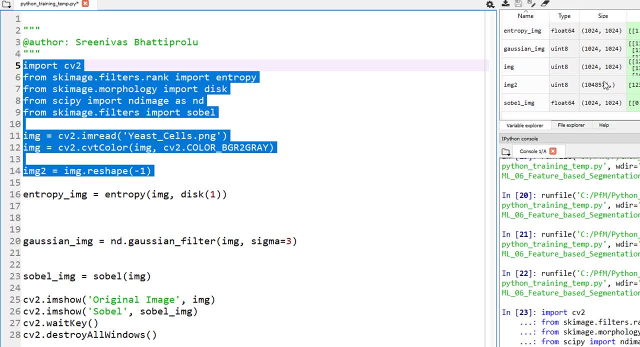 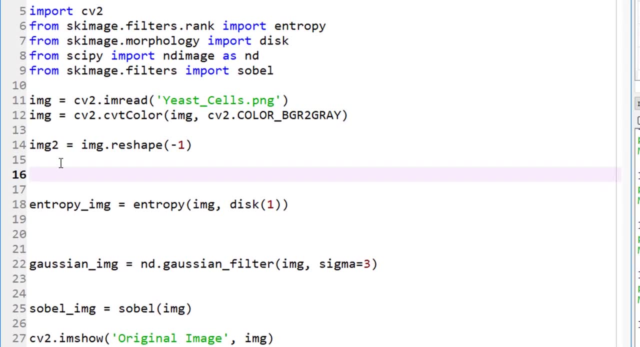 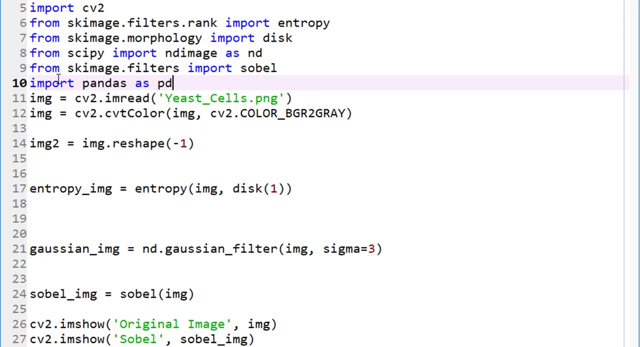 this matrix and then converting that into one single array. so now that we have it, okay, let me create an empty data frame. okay, again. well, did we import pandas? let's go ahead and import that. import pandas as PD again. if you haven't, if you don't know what I'm talking about, then you haven't. 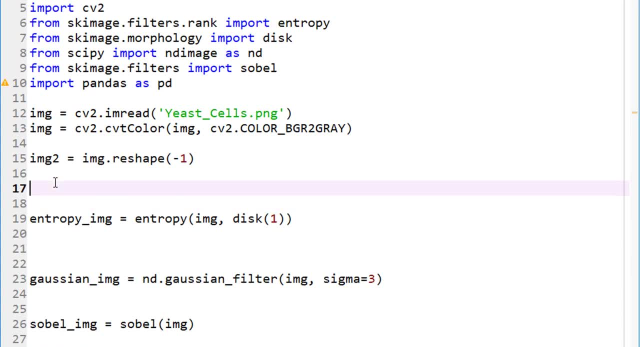 watched my pandas tutorial, so go back and watch the tutorial video, but again. so I'm going to create a new data frame. okay, equals to P D. again, we know how to define a new data frame and I'm going to define an empty data frame. so now, 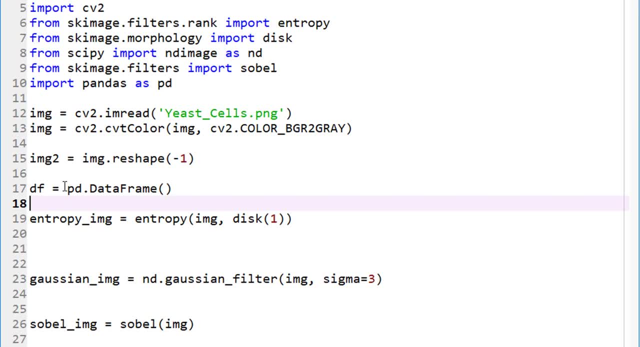 I have a, an empty- think of this as an empty excel sheet that I plan on filling it okay with the data that we are going to generate. so right now we have empty one and the first data, first column. remember, if we go back to our image, for example, this image, right? so first of all, what's defining? 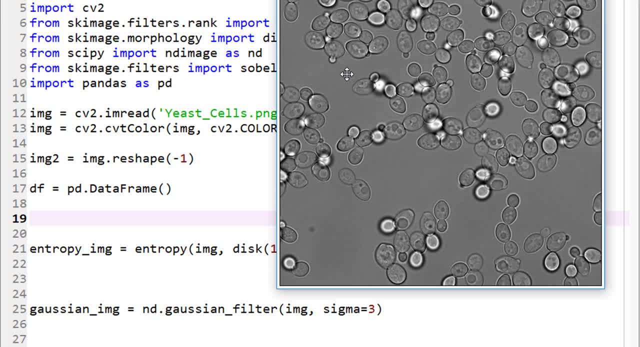 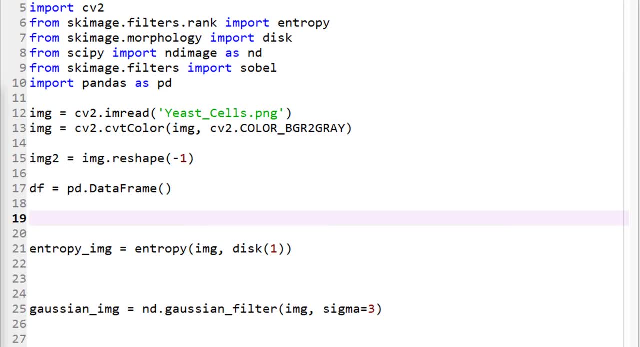 this. I mean I'm going to go back and I'm going to go back and I'm going to go back and I'm going to create a new window for us on the Chromium. so I'm going to go to the search bar and I'm going to create a new XML slide case, this one slice. 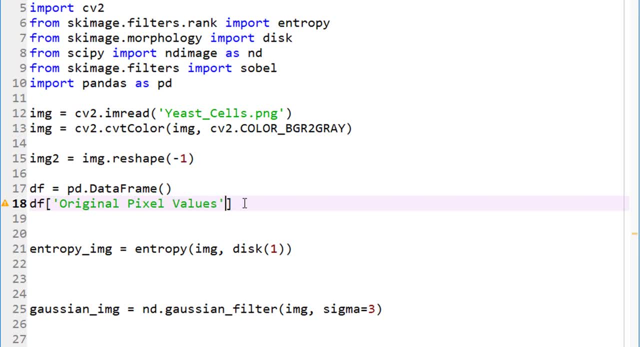 add a new. I'm going to call this text cutout file listener and I'm going to call this stuff right here, family Ado and fill it with what Image 2.. That's it, okay. So if I run this again, if I run this, 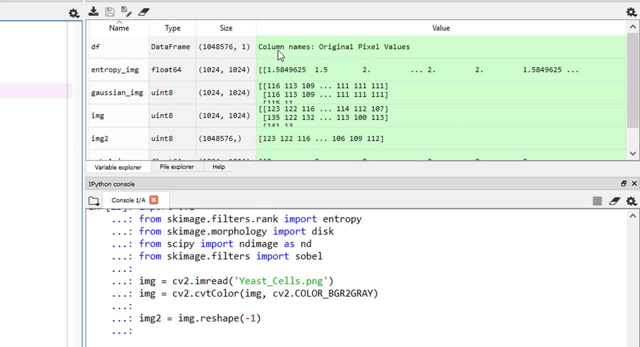 you should see my data frame. here is again. I have a column name called original pixel values. okay, That's my single column right there, and I have 104,, 8,, 5,, 7, 6 entries in there. 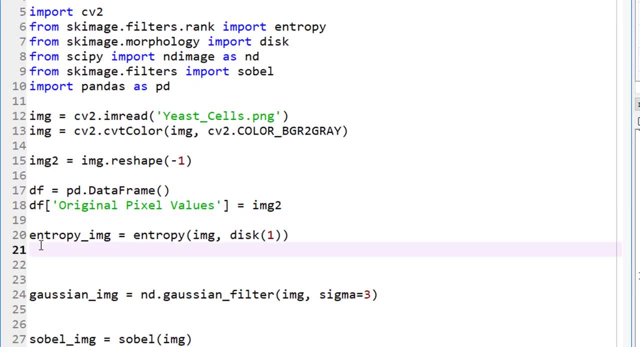 Now I need to add another column. I think you got the idea here Now that I'm calculating entropy here. okay, So let's go ahead and first of all unwrap the entropy. Remember, this entropy underscore image is a 2D image, so we need to unwrap that. So I'm going to call this entropy1. 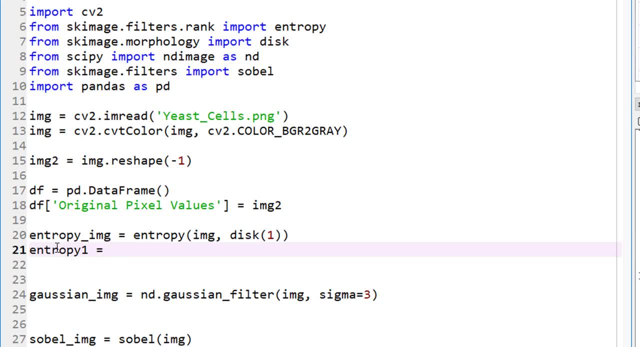 equals. okay, And this is what did we call Entropy underscore, image dot reshape. We are doing exactly the same thing we have done with our original image, so I'm reshaping this, so it is again 1.. And now I can go ahead and add it to our data frame, and I labeled my data frame as df, That's. 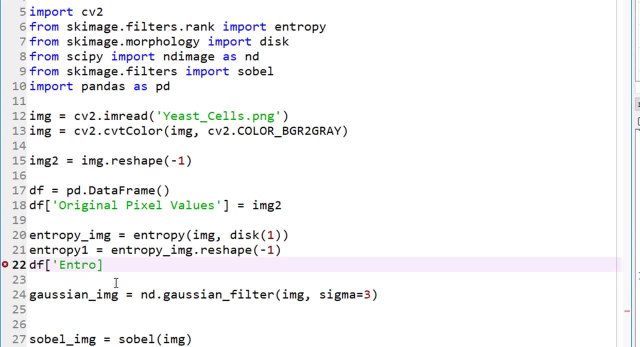 why I'm doing df here. okay, And the new column name? I'm going to call it entropy, and what is it equal to Entropy1.. That's pretty much it. So, for every one of these filters, go ahead and do. 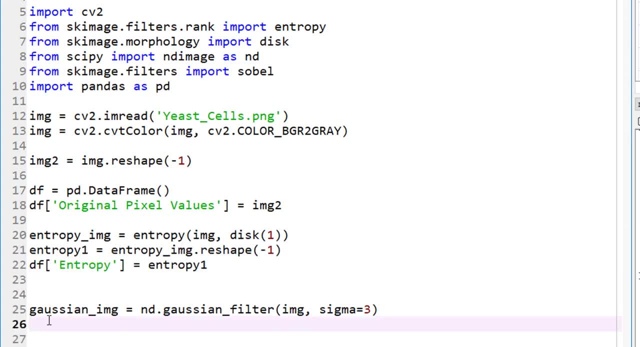 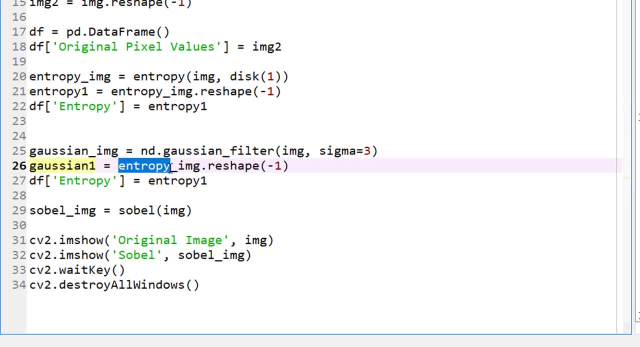 that and because I'm a bit lazy, let me copy that right there, paste it and change this to Gaussian 1. And nothing. but if you copy, make sure you change everything that you should be changing. I made this mistake a bunch of times, where I forget something and then it takes forever to figure out. 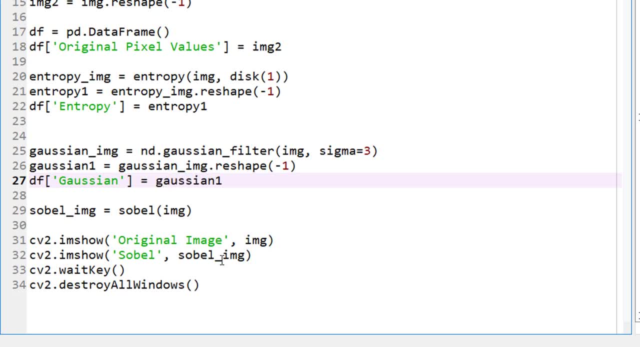 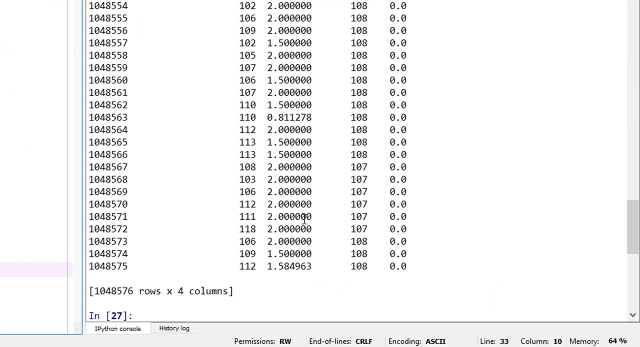 why things are not working the way you expect them to work. So I think this works fine and let's do this one final time for my Sobel filter. So my Sobel1 equals to Sobel underscore image, and this is my adding a new column called Sobel and then Sobel1, okay, And let's not visualize any images. We have done that already. Now, when I run this, if everything works fine, that's good. That's a good sign. okay. Now let's look at how our data frame looks like and we can do print. You can do the entire data frame. Let's go ahead and do that first, okay? So when you print this entire data frame, you should see a whole bunch of values right there. 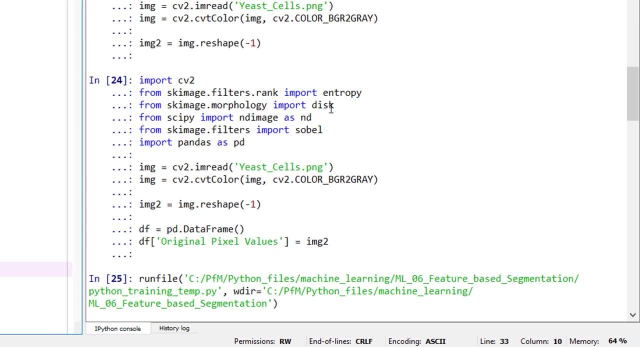 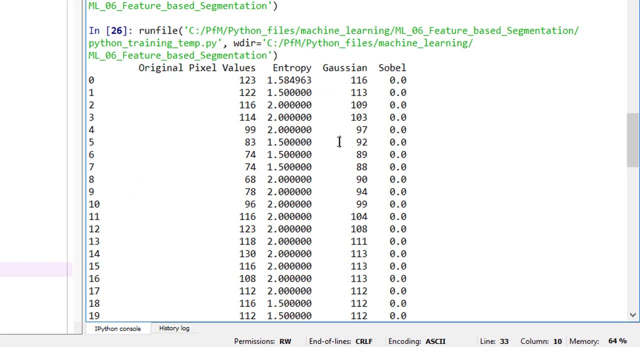 Okay, it shows that these many rows, four columns and, if I go all the way to the top, original pixel values, entropy, Gaussian, Sobel. So these are the values. So these are individual feature vectors at every pixel. That's pretty much it. So now our data frame is ready to go into a machine learning algorithm, yeah, where it can train and create a model. okay, So one feature that I did not show you. 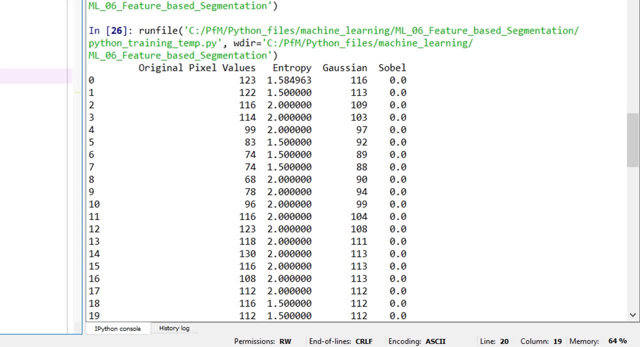 which is my most favorite feature of all time because it turned out to be so amazing in a couple of situations. for me It's called Gabor filter- G-A-B-O-R- Gabor filter. This can be so useful, especially if you are, for example, looking at features that are oriented in a specific direction. Let's say you are working on images that are, for example, from sedimentary rock and you know, for sedimentary rock, the features, the bedding layers are.